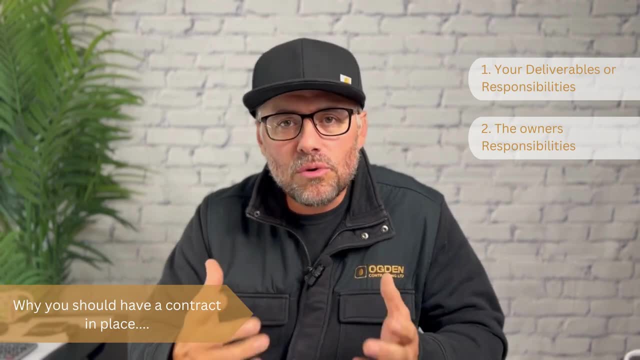 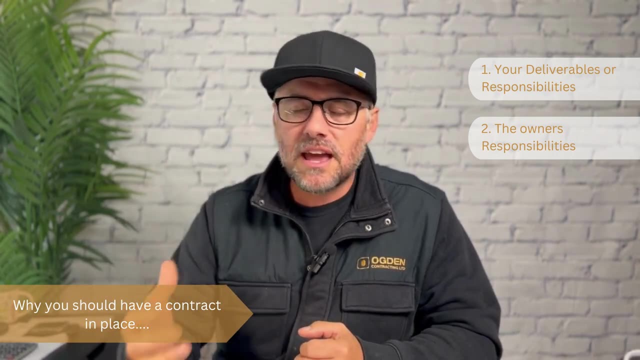 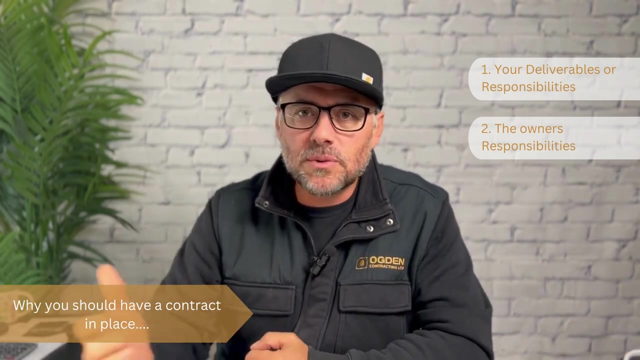 what you're providing them. Number two: the owner's responsibilities. What is the owner going to provide? You don't have a crystal ball and you can't read mine, So the owner has to tell you their vision Along the way. if they don't like something, it's their responsibility to come to. 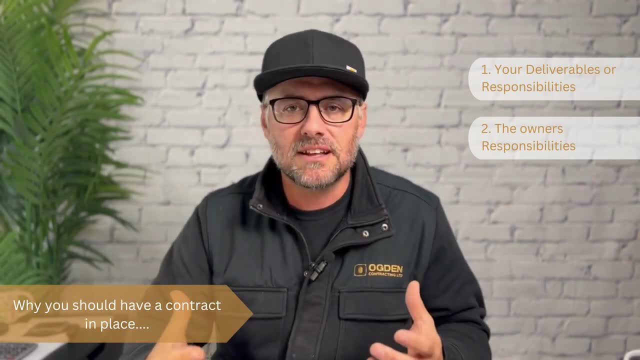 you and tell you what you're providing them. So if you're providing them a whole renovation, it's their responsibility to come to you and say, hey, this isn't being built the way that I envisioned it. But if you could write those contracts in place, that that's the owner's. 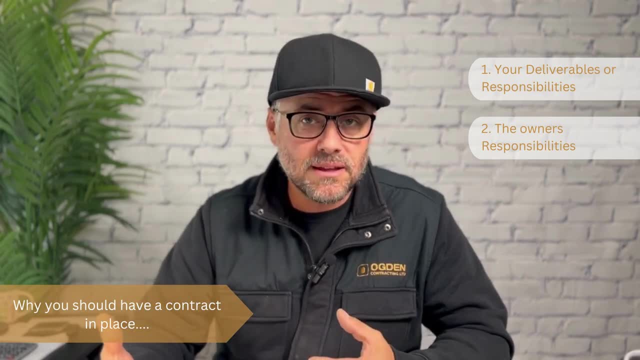 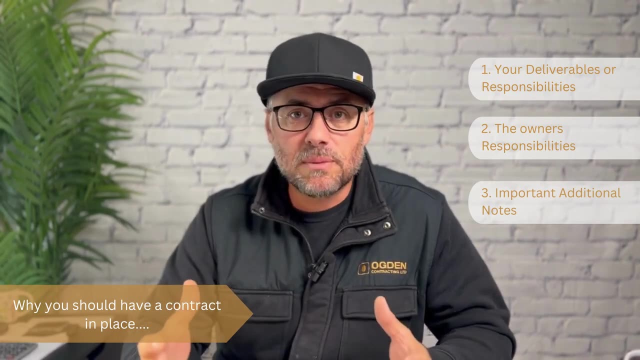 responsibility that they need to be proactive during the job. This can help a lot in the long run. Number three: additional notes. So I always tell my owners: if you want something to be saved, let's say we're doing a renovation and we're going to be tearing down this wall, but you want 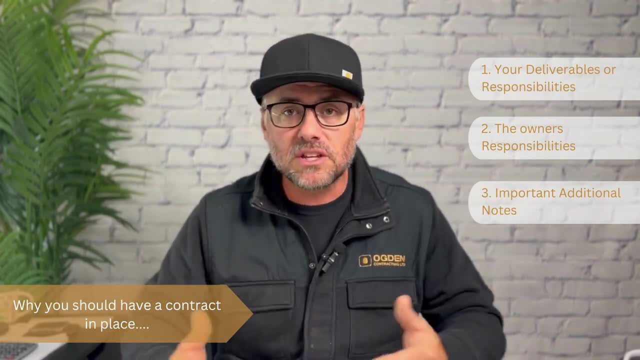 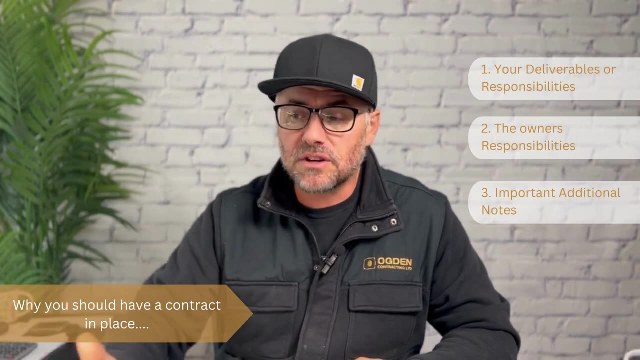 that plant or you want, you want this fridge or some appliance, write the word saved on it, because you telling me you want to save that. And then I have to tell my project manager, and then my project manager has to tell the site super and the site super has to tell the staff. 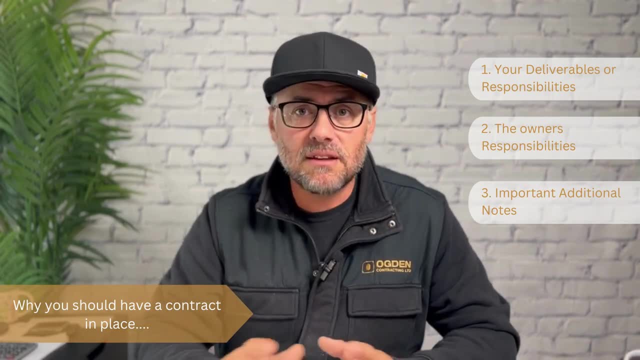 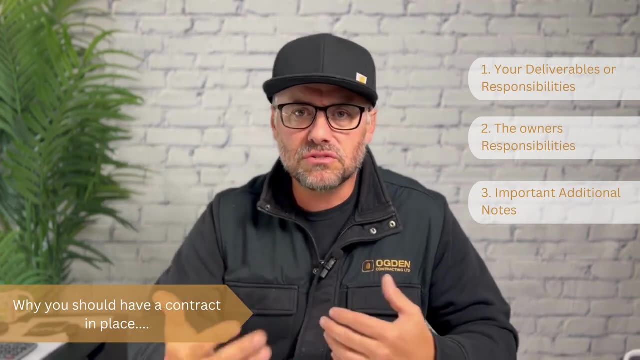 somewhere along the line it's going to get misconstrued and people are not going to get the picture clear, So they need a clear sign that says saved. So there's additional notes that you really need to put in there. If a homeowner is living in a house, well, 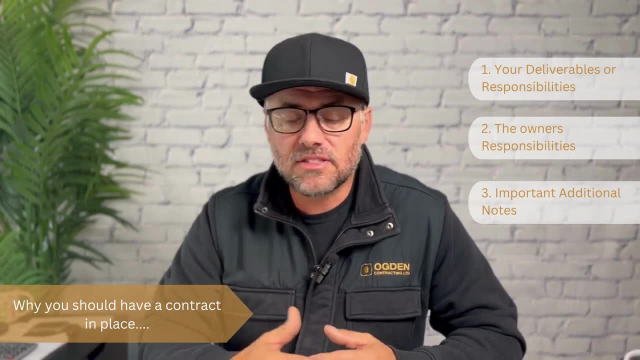 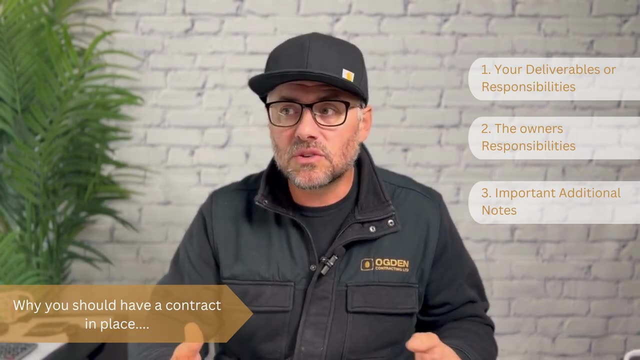 there's dust. So you need to make that aware to the owner, that there's going to be dust, Because there's been so many times where the owner has come to me and said: I can't stand all this dust And I said: well, I told you it was going to be this way, But if you have it in writing, 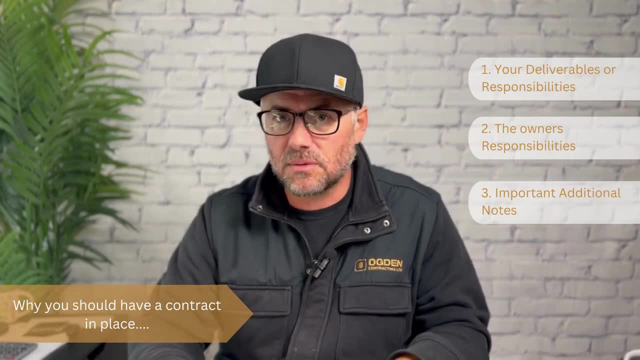 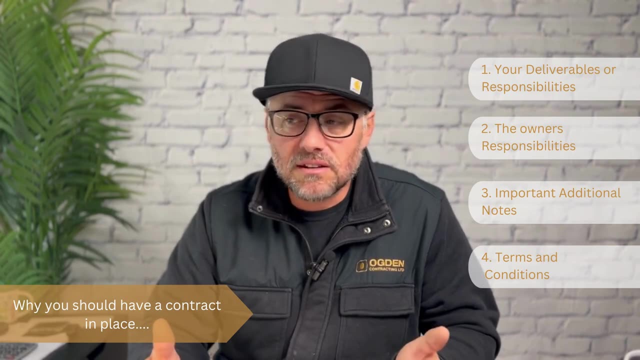 they know they can look back and go. oh yeah, he did actually tell me that. Number four is your terms and conditions. What are you going to do once the job's done? Are you going to just they have to look after all the warranty issues, or are you going to provide some sort of warranty? 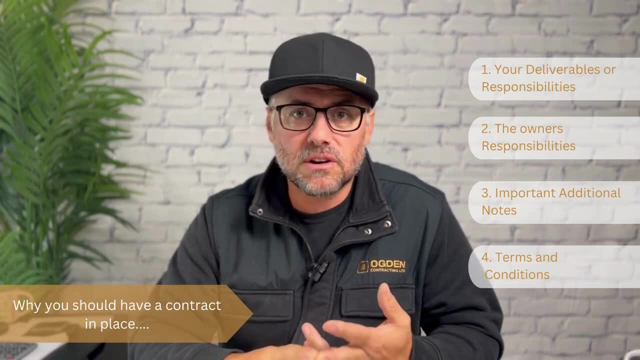 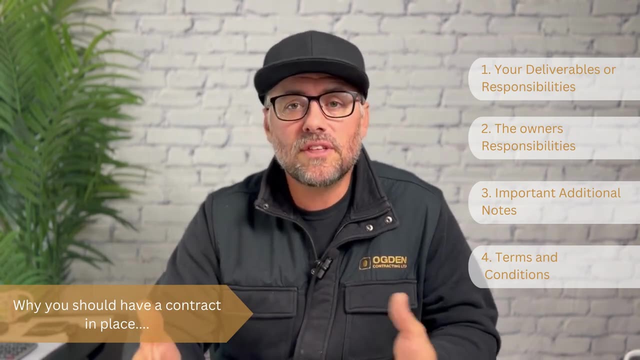 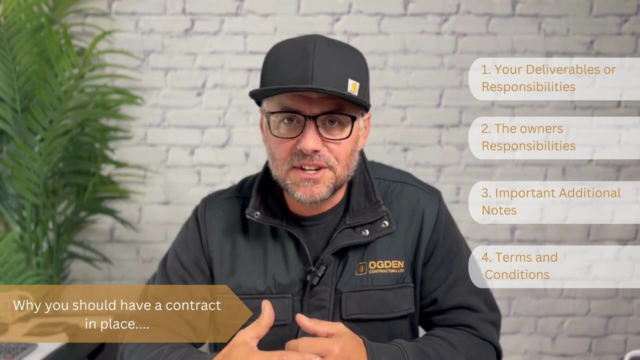 quality control checklist, making sure that the products are working properly and that they're looked after. If there's a problem in the future, they want to know that they can come to you and you provide a service that'll look after them, And this is part of why we need to write these agreements. 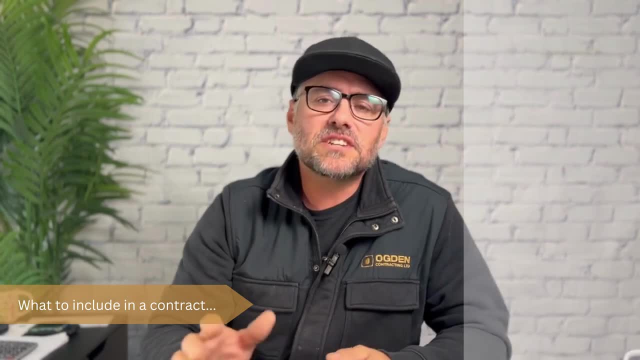 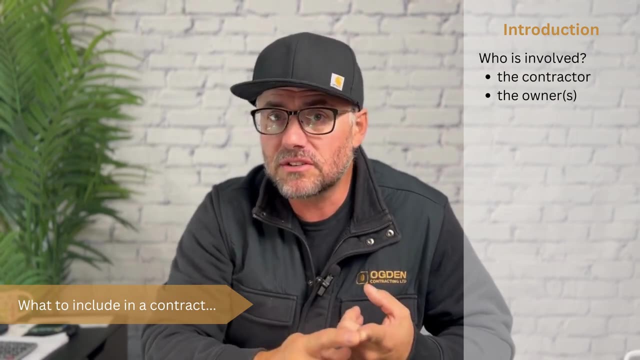 So here's some things that I include in my contract. The first thing I start with is the introduction. This kind of introduces who's involved in this agreement. So it's going to be me, the contractor, or you, the contractor, and the owner. So I'm going to start with the 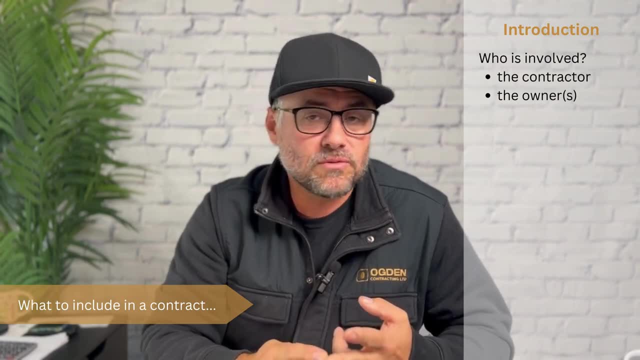 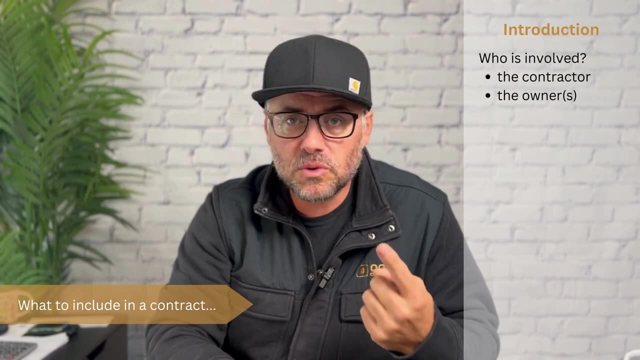 the stakeholders, which are the owners. So if there's more than one owner you want to include, let's say, a husband and a wife or a partnership, or maybe there's only one person, but everybody that's part of the stakeholder needs to be written in this agreement: Anyone that's going to be. 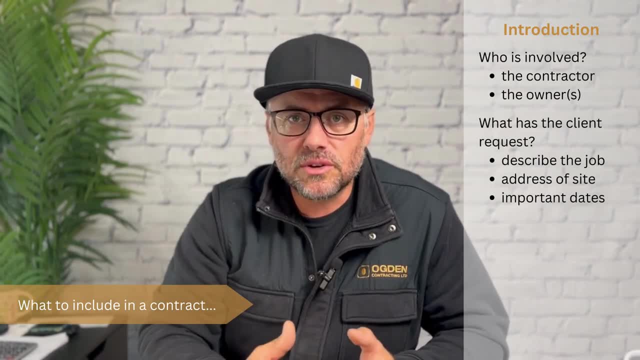 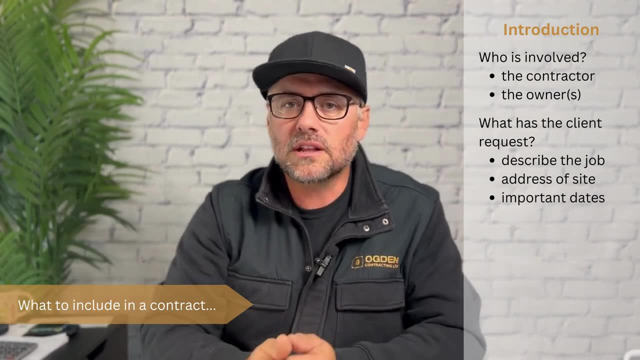 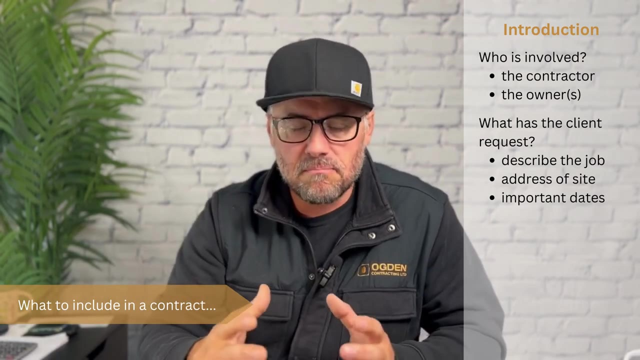 making decisions needs to be written in this. You also want to include what the client has requested you to do, such as the client has requested me to renovate this building, or the client has requested that I build them a house On this particular land, And you always want to include at minimum the address of the job that 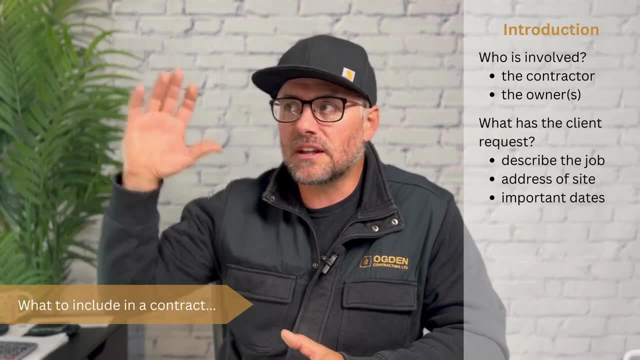 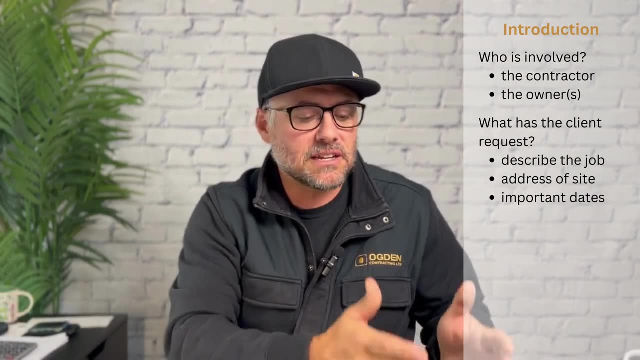 you're going to be working on, So it's clear that you're not doing a renovation on a different job site. If this ever went to court or you wanted to have a dispute, it's written on the agreement. It's clearly that this is where the job is And I always write out the purpose of the contract. 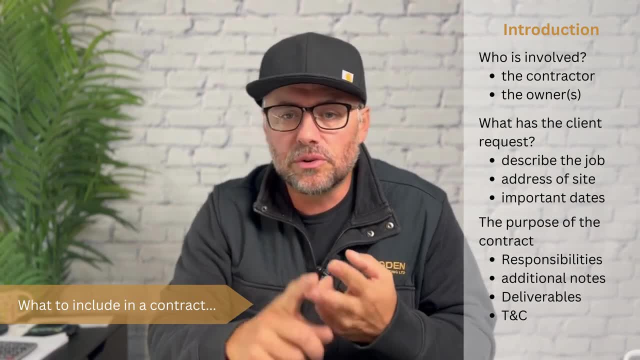 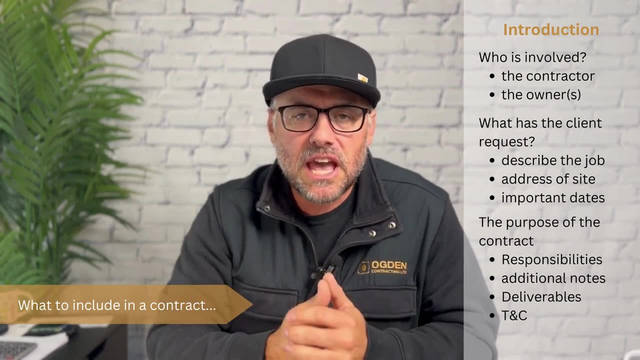 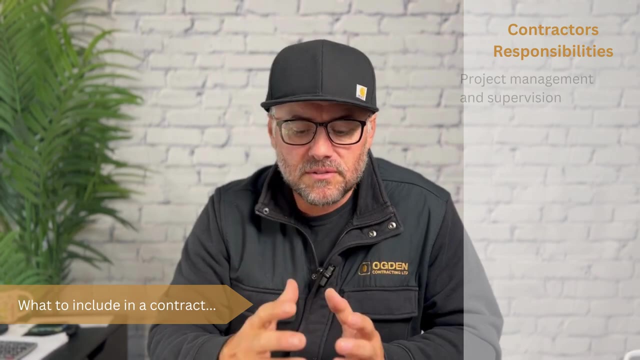 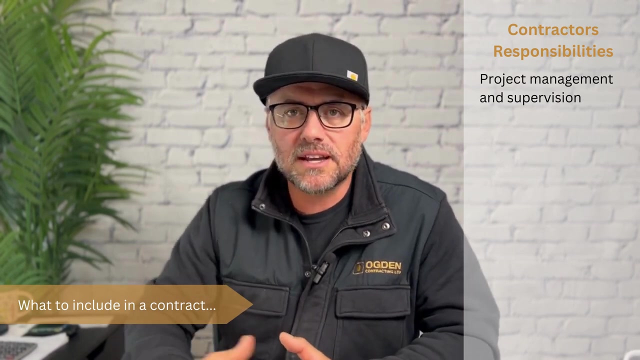 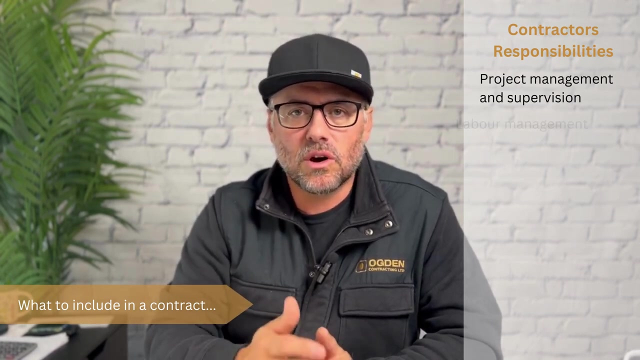 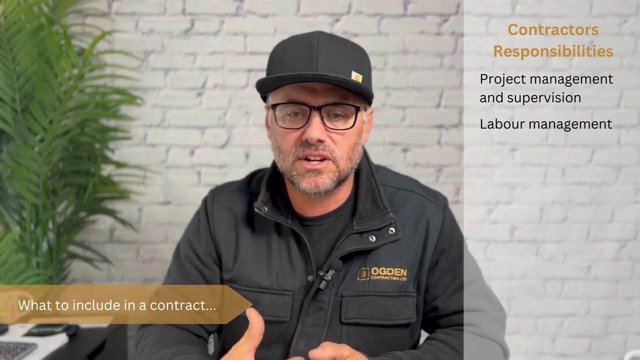 It's the why. So the contractor's responsibilities, the owner's responsibilities, the We're also labor management. We're managing the labor on that job site as well. That's not the owner's job to manage, that, It's the contractor's. 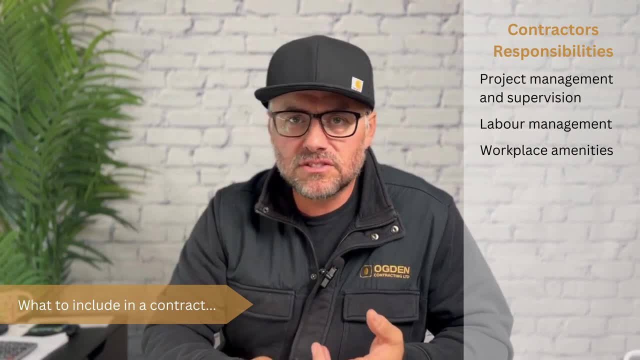 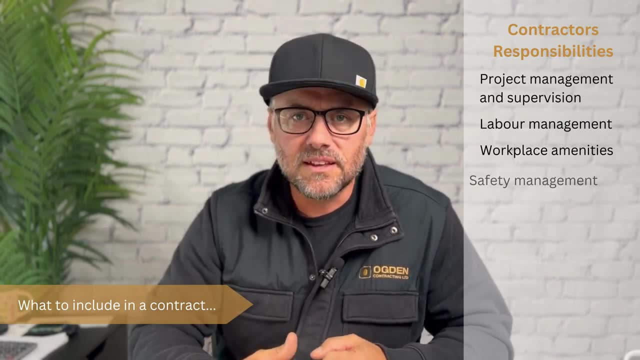 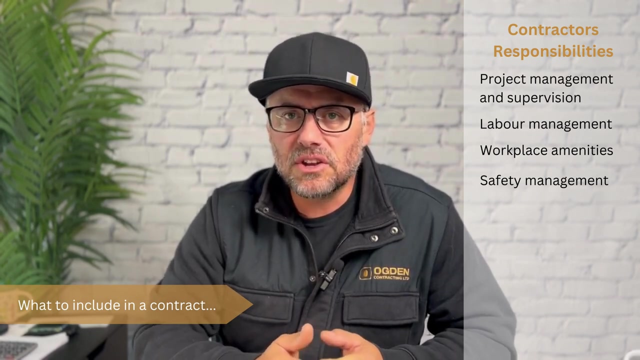 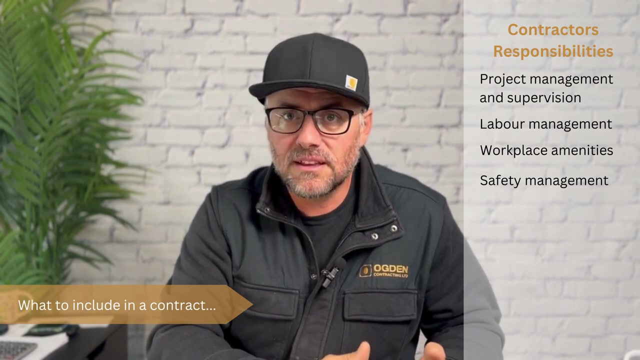 Workplace amenities. So we provide toilets, fencing, security. We're going to include that in the contractor's responsibilities- Safety management. It's your responsibility to go to WorkSafe and file a notice of construction. This is so that WorkSafe is aware that the job sites are being done safely and 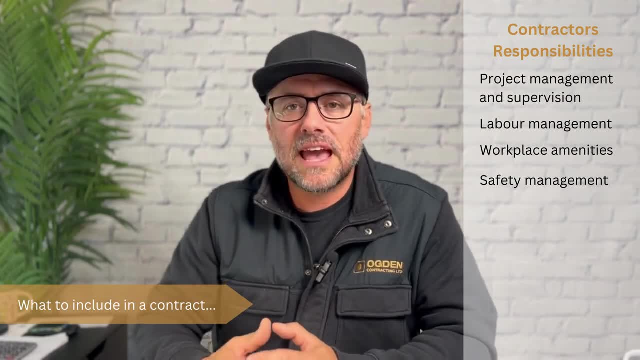 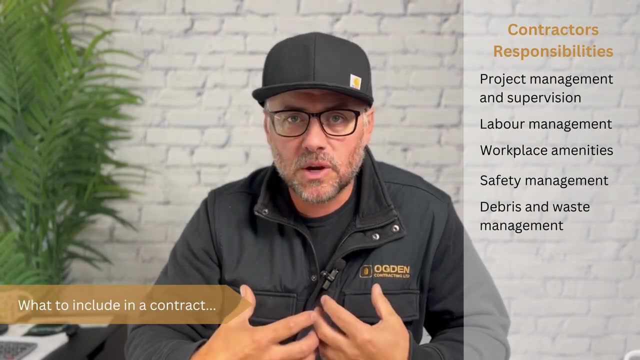 for the health and safety of your staff and the owners on the property. Debris and waste management is another one You're going to be responsible for- or I'm responsible for- getting rid of all the scrap and all the debris on the job site, Also during renovation. 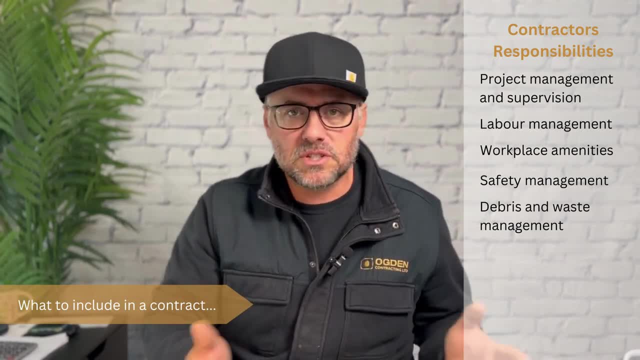 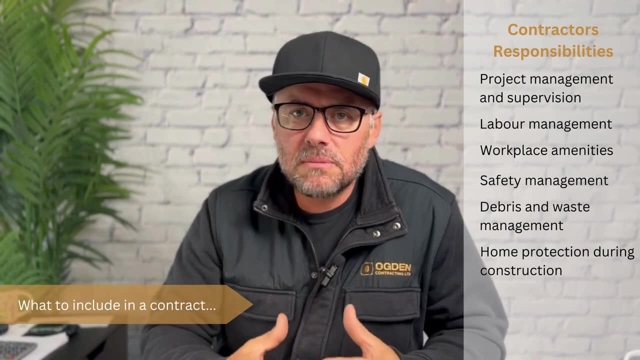 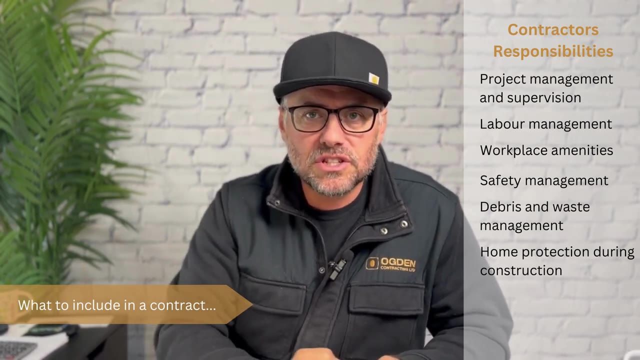 there's going to be some hazardous materials perhaps that you need to dispose of in a legal fashion. Home protection: The owners need to know that you're going to be responsible for protecting their home. You can't be dragging cords or things across the brand new floor and scratching them up, or 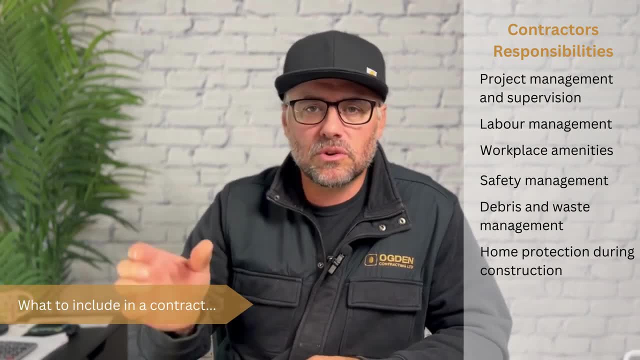 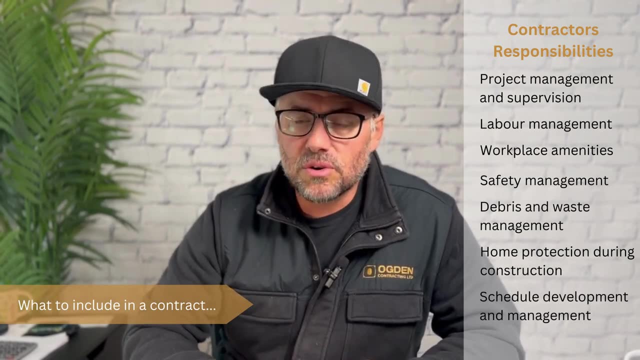 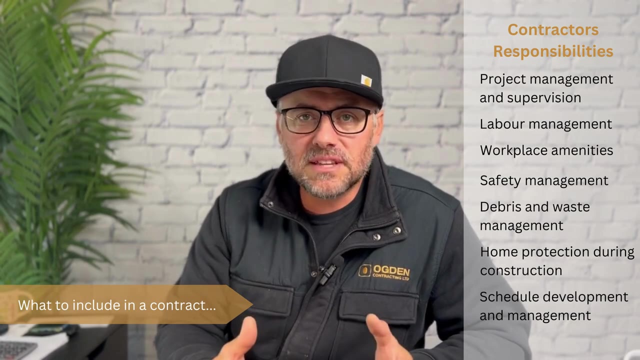 digging up their corners, So they need to know that you're protecting those with either a corner wrap or floor protection. Schedule and development: It's very important that the owner knows when your start date is and when you plan to finish. This is one of the biggest things in construction. 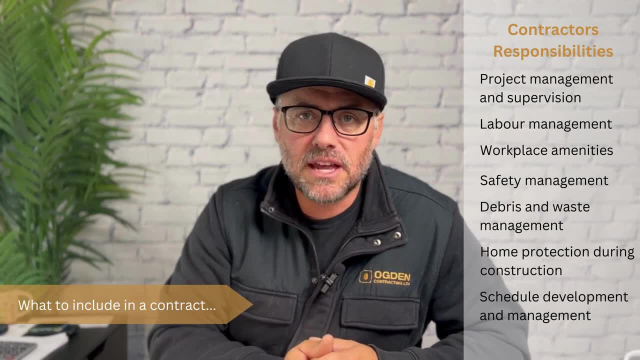 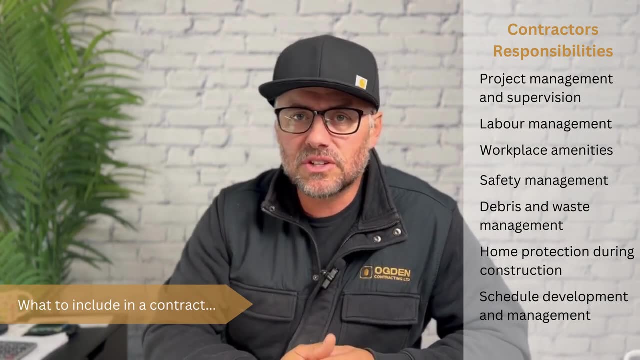 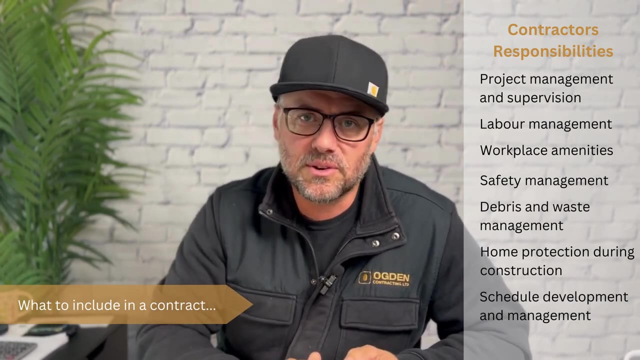 that owners are most frustrated with is there's lack of communication. When is this job going to be done? People always ask me that How long is, because the last time we had a contractor, it took months and months longer than we expected. So you have to be able to provide a schedule for. 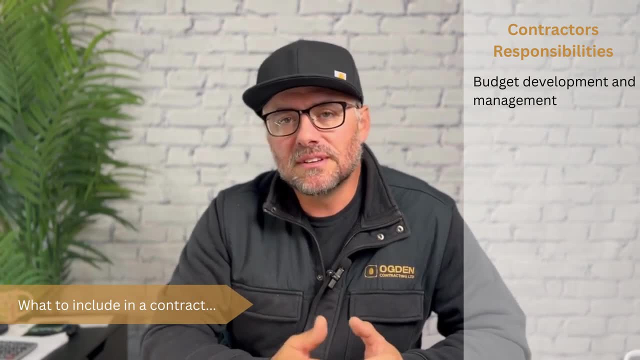 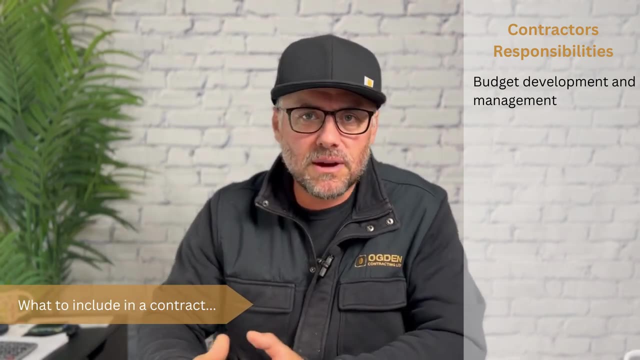 the owner Budget development and management. So, yeah, it would be nice if someone just had an unlimited budget, but I always design a budget for my owners so that they know exactly where to put their money If one job goes over in budget. 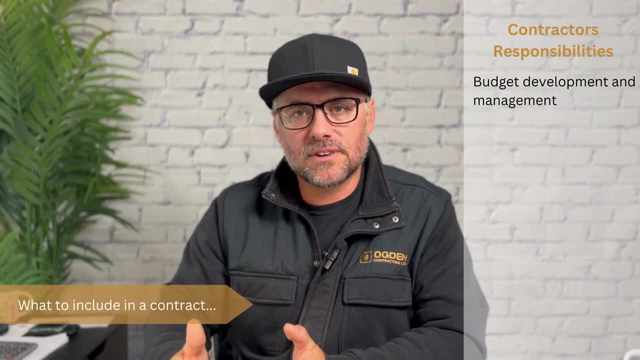 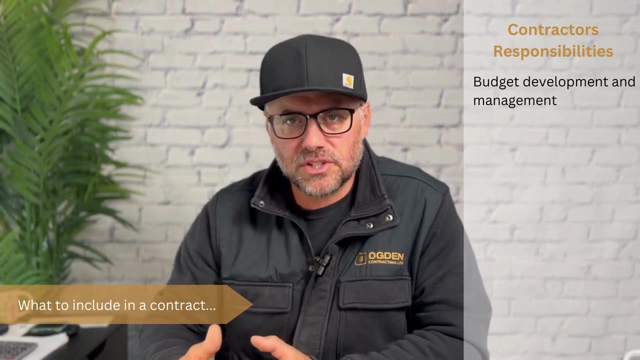 if they're really tight with their numbers, then maybe we could look for savings on the next one. And it's also very good to provide your owners with updated budgets as well, on a monthly basis, so they know where they're sitting with their budgets. Material and equipment installation. 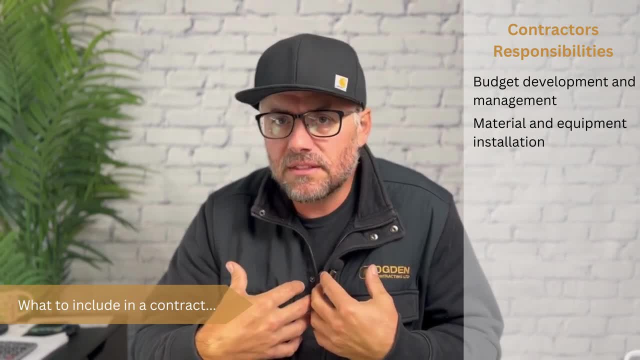 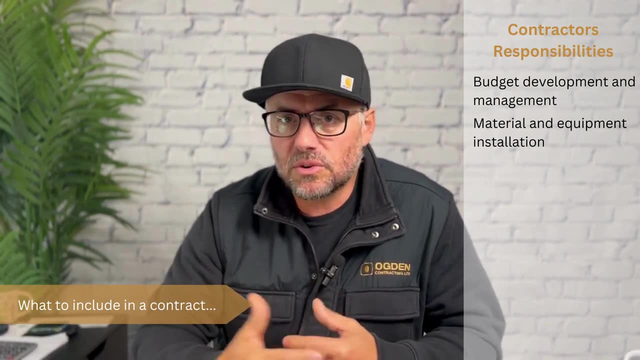 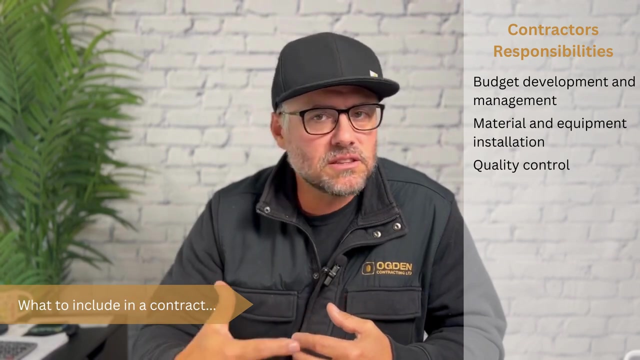 So I'm going to be the one installing the fridge and all the equipment in the house. We're not going to ask the owners to do it. So we want to provide that as our responsibility, so that the owners understand Quality control. It's our job, It's the contractor's job to look at the quality. It's not the owner's job. 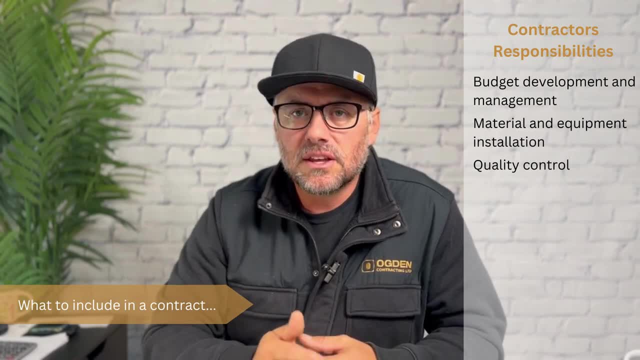 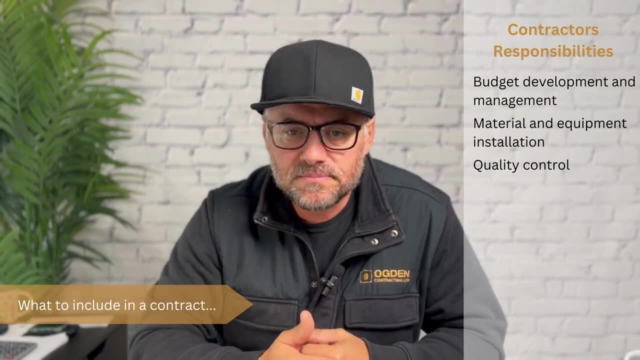 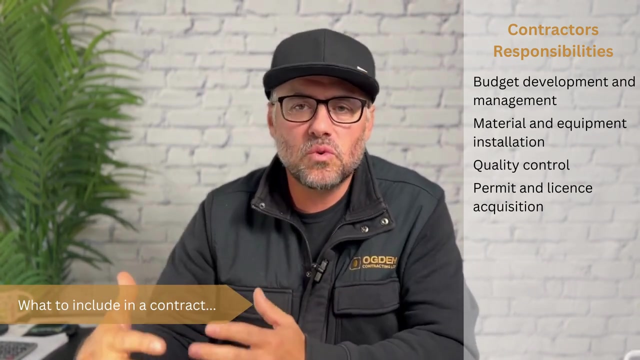 to point out the flaws. It's our job to point out the flaws. It's best to get to that before the owner even sees it, so that they know that you're being proactive in the quality control, Permits and licensing. So you are responsible for providing the city with your business license. 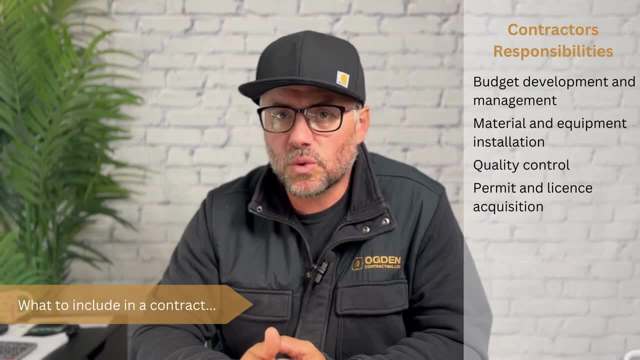 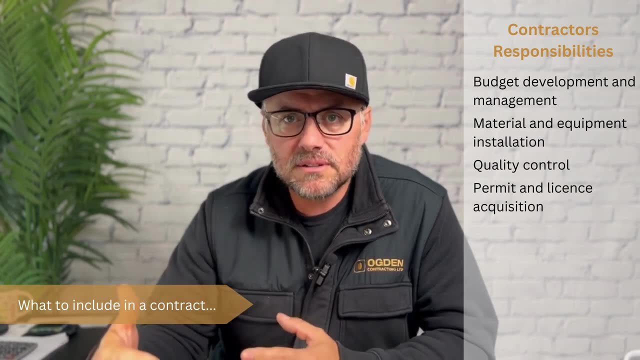 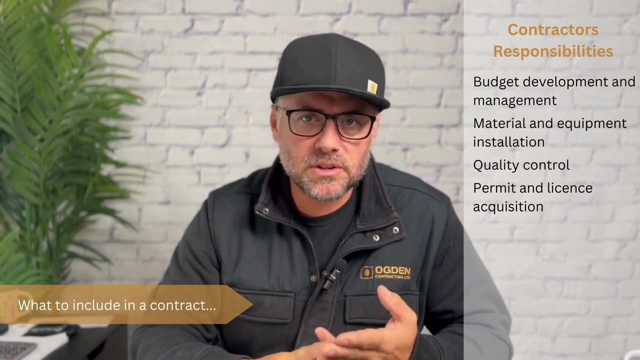 as well as all the business licenses for all the subcontractors working on that site. It's not the owner's job to do that, It's yours. It's also your job to apply for the permits, receive the permits, meet the inspectors, book the inspections and take responsibility for all. 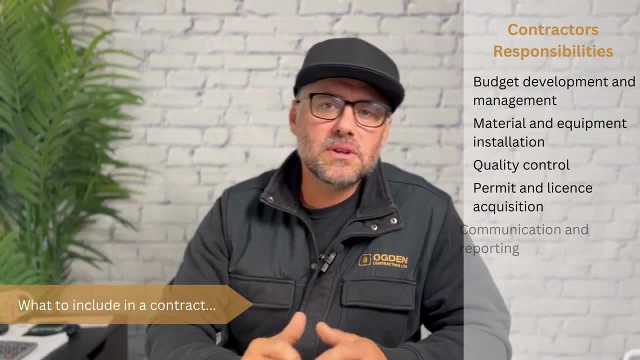 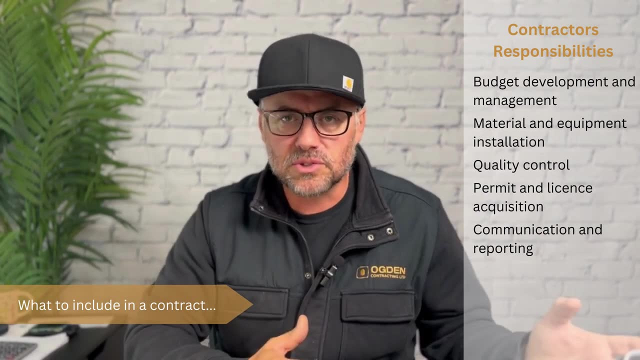 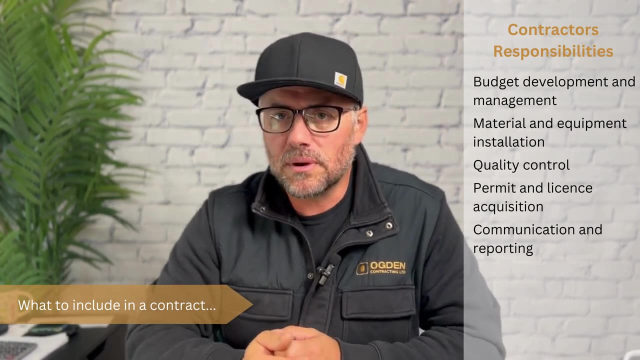 the legal stuff that's being done with the city or community Communication and reporting. It's your responsibility to communicate with the owner if there's delays, if the price goes over budget, if you're expecting something at a different day. This communication really needs to be open. Communication is one of the number one keys. 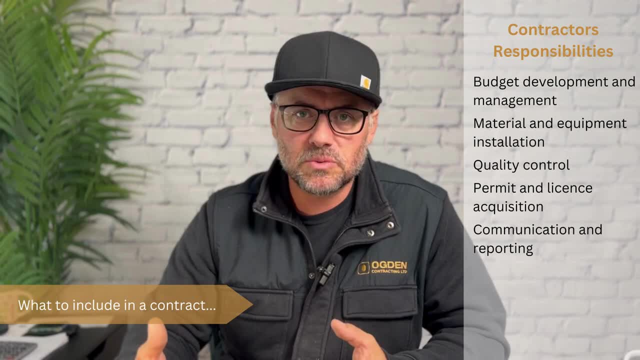 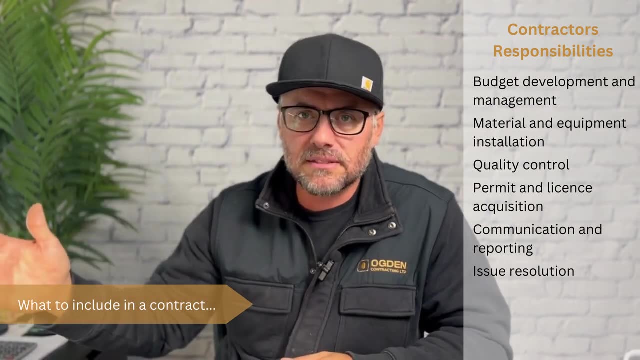 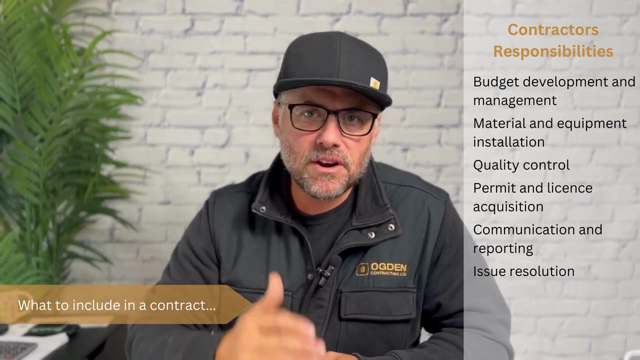 in being a contractor and having good relationships with your owners. Issue resolution: If there is a problem, if your owners say, hey, I did not expect this, what do I need to do? It's your responsibility to resolve that issue professionally and in a 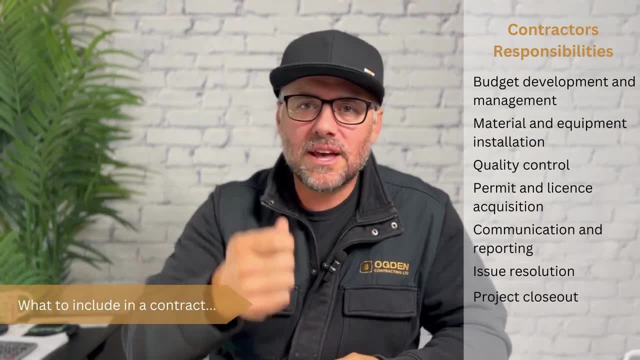 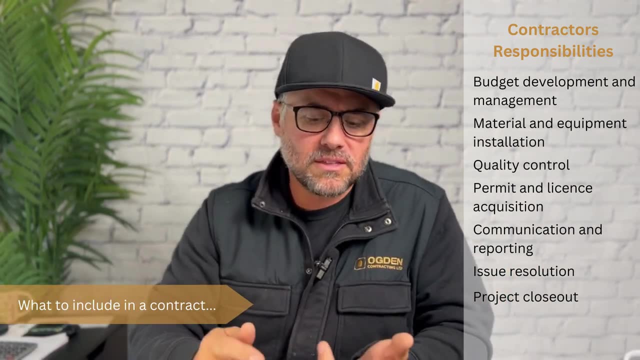 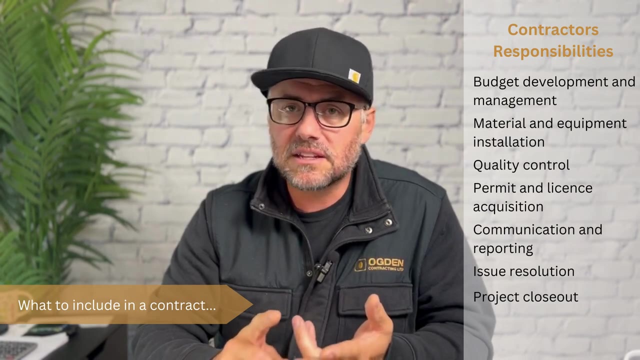 very good tone, manner And project closeout. When you hand over those keys to the owner or you hand over the job and say we're done here, you need to provide them with all the warranty issues for every product that you put in there as well, as I mean I like to include photographs and all the 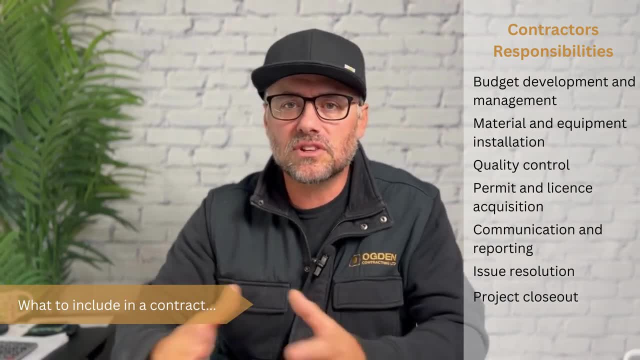 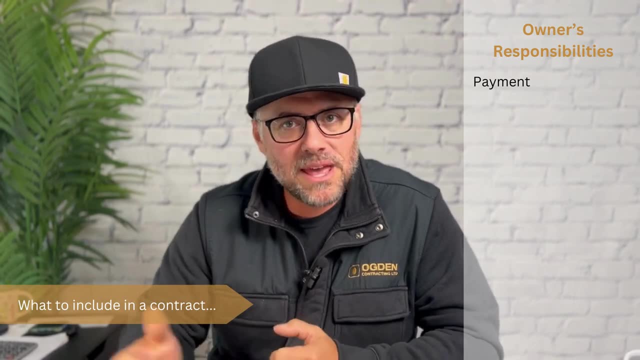 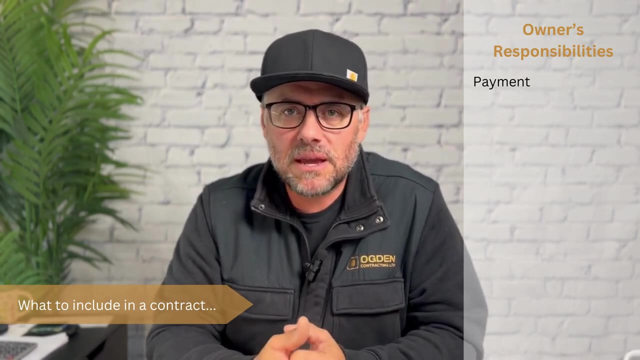 contracts, all the trades that were on site there, so that they have this closeout process. So, moving on to the owner's responsibilities, So the owner is responsible for paying you in a timely fashion, And if you're an owner, you're listening to this and you want to know: well, how many days do I have to pay that? 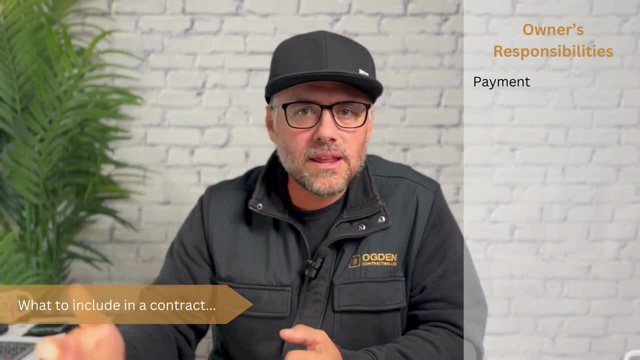 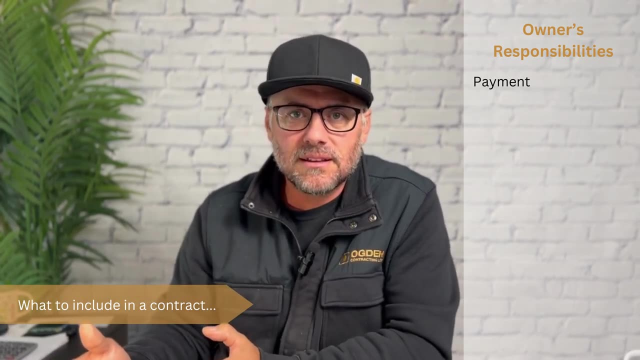 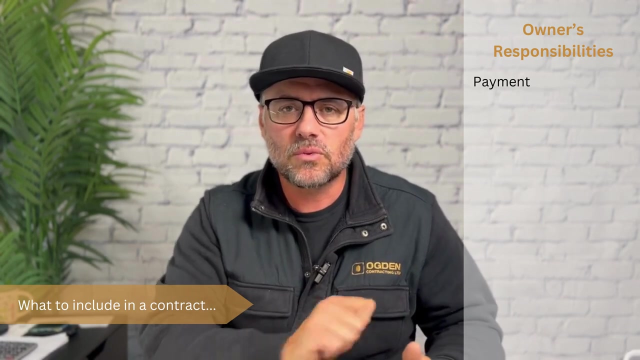 contractor. Pay the contractor right away, Don't wait 30 days, Don't wait 90 days. Pay them right away. They're paying their trades out of their pocket or a deposit And they want to know that the relationship is built on trust. So if they sent you an invoice, write them a check. There's 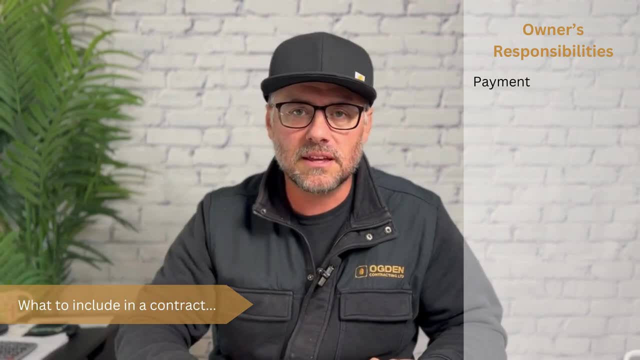 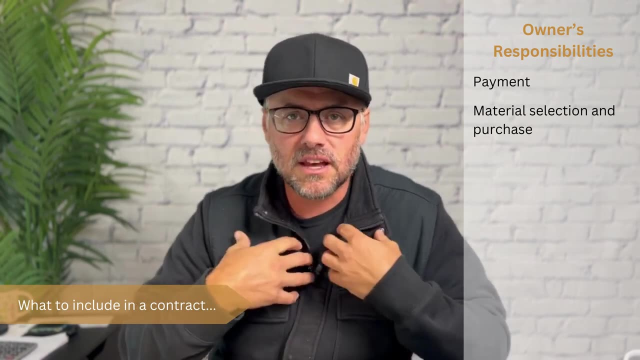 no difference for writing it today, as it would be in two weeks, So write it today. The owner is also responsible for picking out their selection, Like materials, like tile flooring, paint colors. It's not my job. I don't know what you want, So 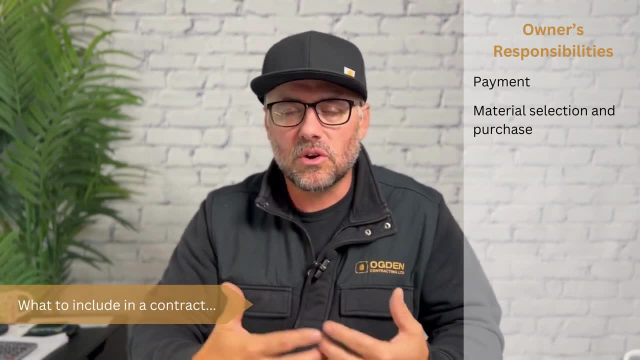 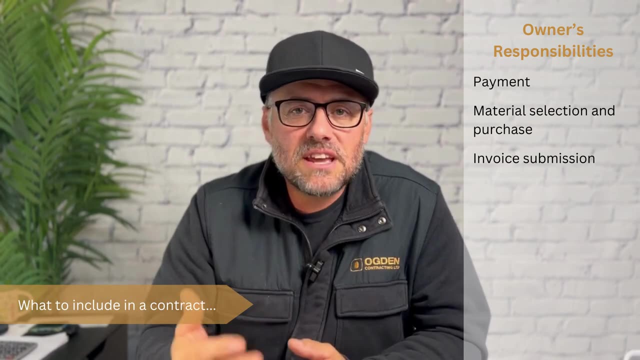 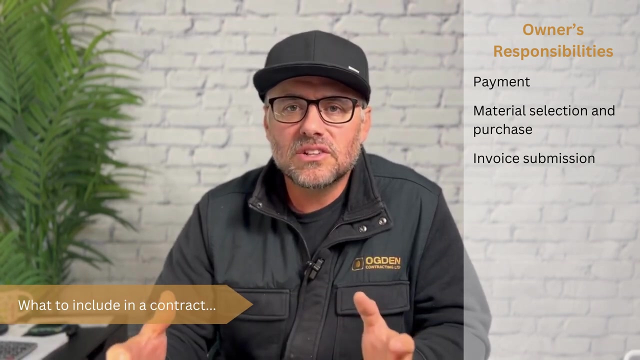 you need to express what you want. The owners are to express what they want and give you the selections for everything that they want to put in their house. Another one is invoice submission. So we base we're- if we're- a cost plus contractor, we base our entire job off of the cost of that. 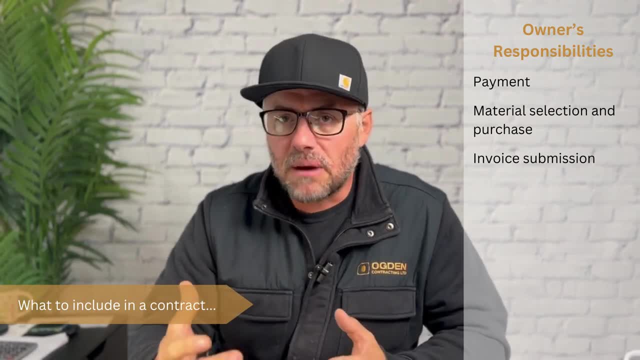 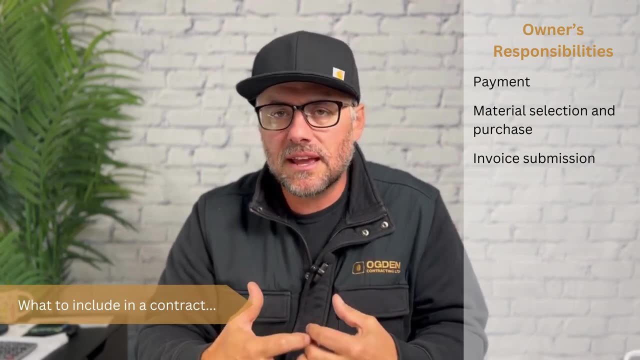 job, We get a percentage of it. So if the owner goes out and buys a product on their own, they should submit the invoice to the contractor. So you should be asking your owners: Hey, I know that you bought some tile. Can you please provide? 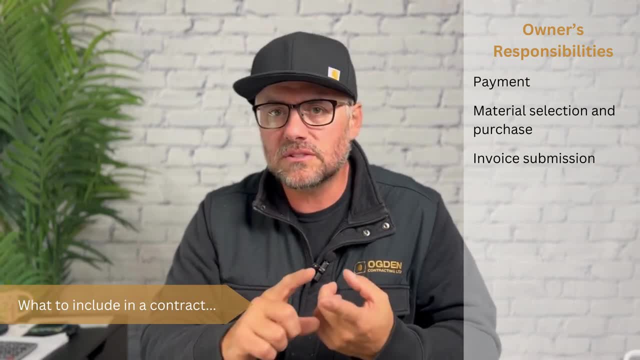 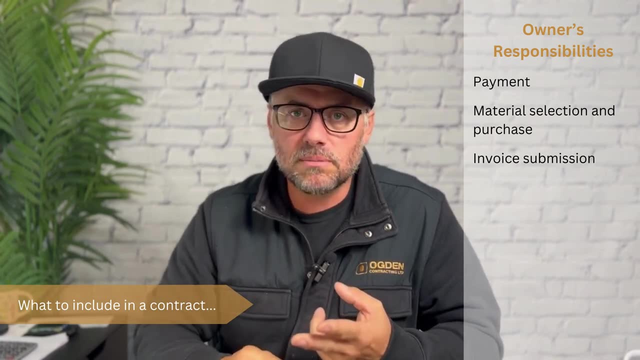 me with those invoices. There's lots of reasons why. one is we like to keep track of what products we put in the house to. a lot of contractors work on cost plus, So that's part of the job cost. There's also some warranty issues in there as well. We're going to be taking care of the. 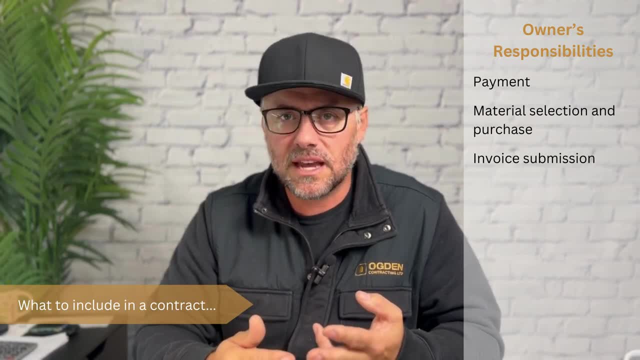 warranty. So we want to know what products you bought and where you bought them, So we can look at what products you bought and where you bought them. So we're going to be taking care of that. Another responsibility of the owner, which is very important, is being available for communication. 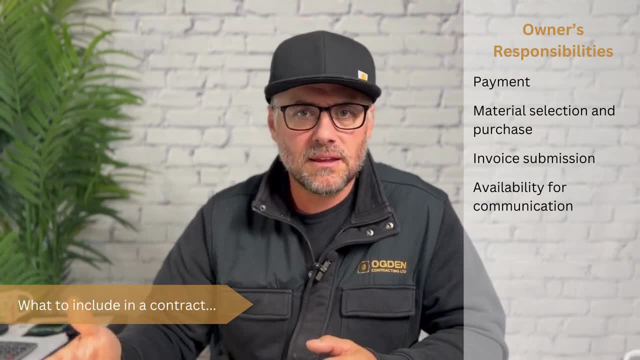 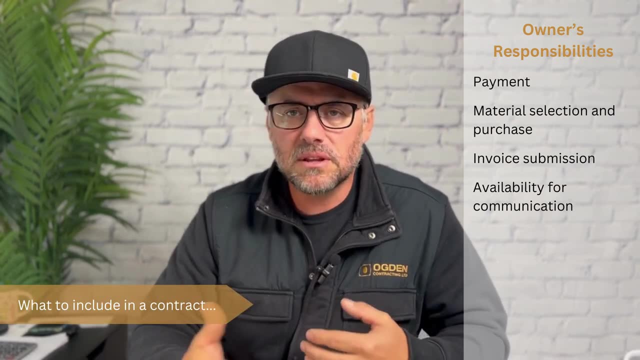 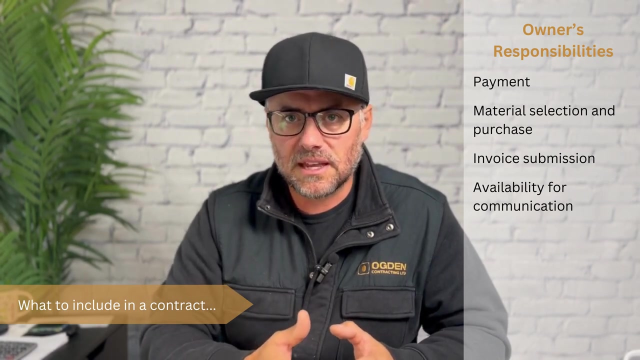 If the owner's only available Sunday night at midnight, how is the contractor ever going to work for you? How is a contractor ever going to be able to communicate? So it's best that you set a day that you both can agree on, once a week that you can, that you like an hour or two. 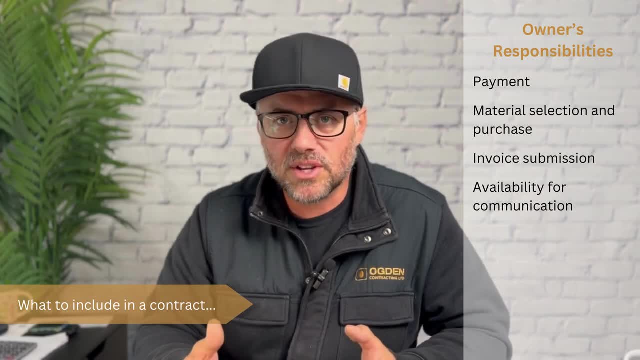 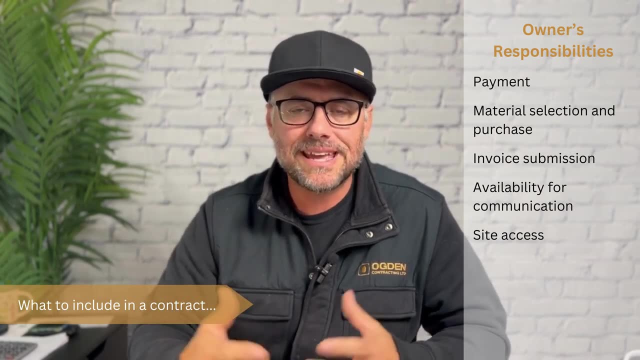 where both of you can meet and communicate what's happening on the project. Another one is site access. If we're doing a renovation for you and your doors are locked and we show up there at seven o'clock and we can't get in, that's not good for the contractors. Our sub-trades are charging us by. 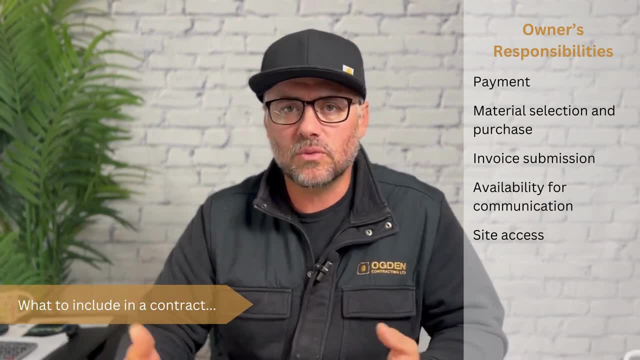 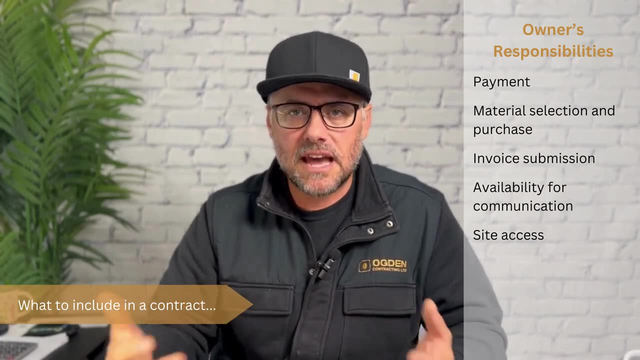 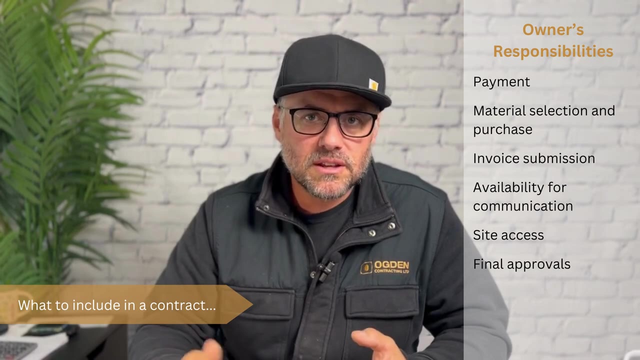 the hour at that second. So you need to provide site access. whether it be through a gate, a gate code or a key to your house, the owners need to provide site access. The owners are responsible for final approvals as well. If there's a product that you purchased and we're going to sign off on it, 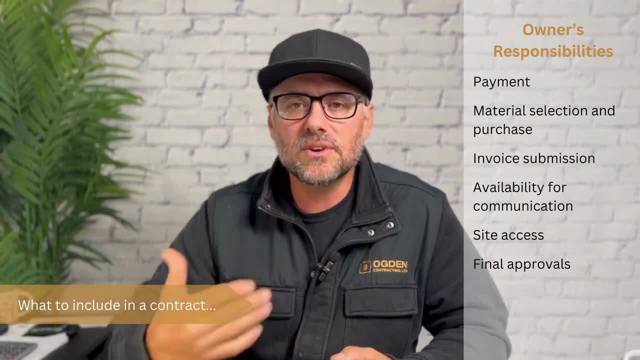 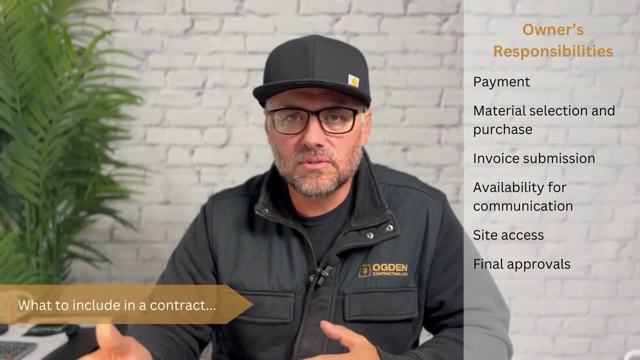 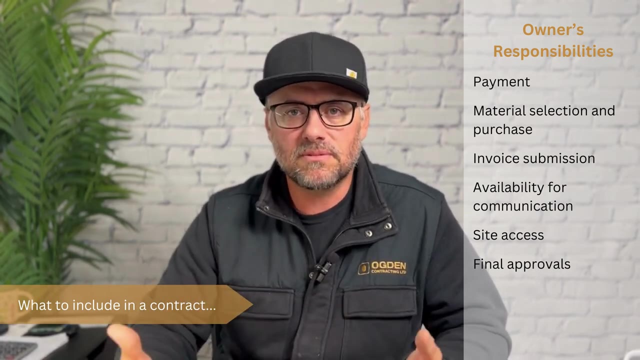 you need to sign off on that final approval saying that yes, I agree that I'm, this is the product I want in the house, as well as doing the final approval on the job once it's completed, You need to go through the checklist and look at anything that you don't like or something that needs to be. 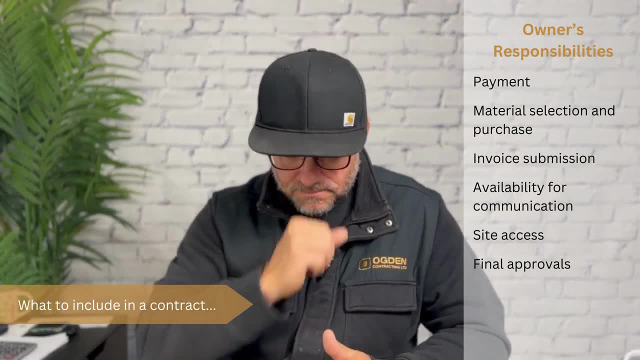 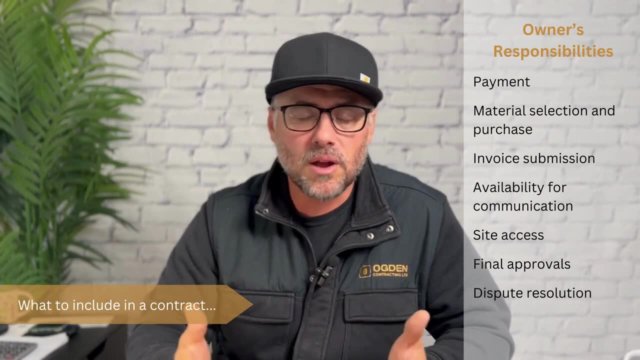 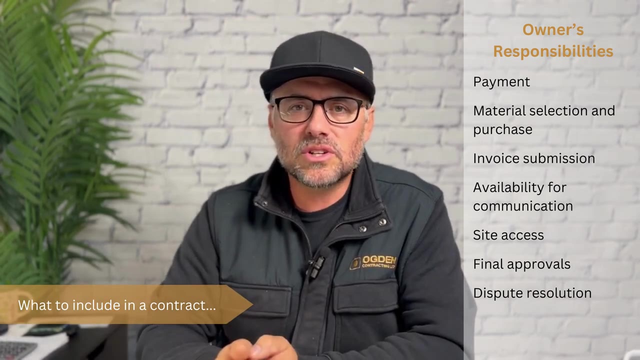 fixed and give the approval. Dispute resolution. If the owner has a problem with something- and I'm going to talk to the owners right now- if you have a problem with the contractor, you need to be able to professionally talk to the contractor. Most contractors thrive on seeing. 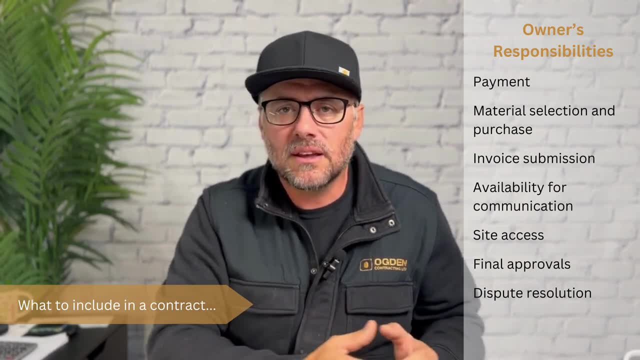 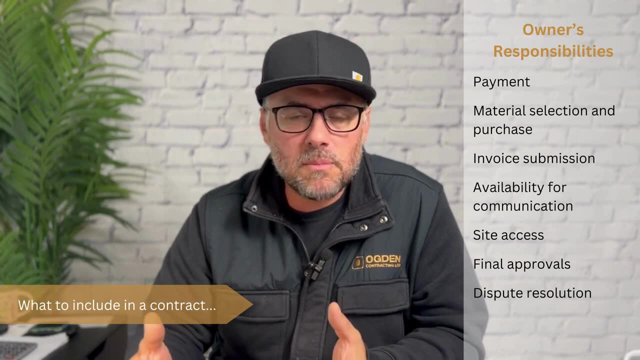 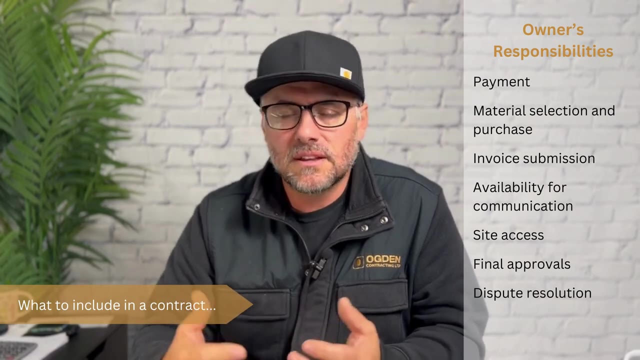 happy homeowners. So if there's something that you're upset about, you need to approach the contractor in a way that you're not creating an unsafe environment for that contractor. You need to, like voice your opinion in a non-demeaning tone and just ask for it to be fixed. It's very simple. 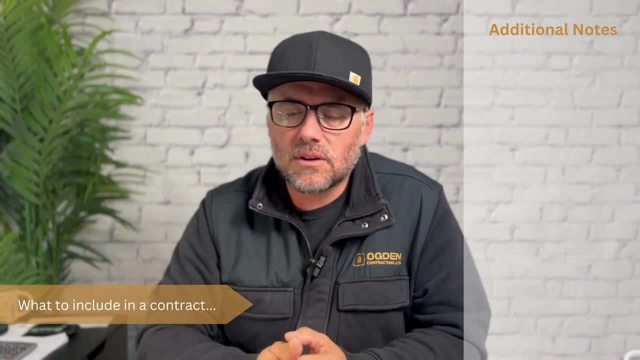 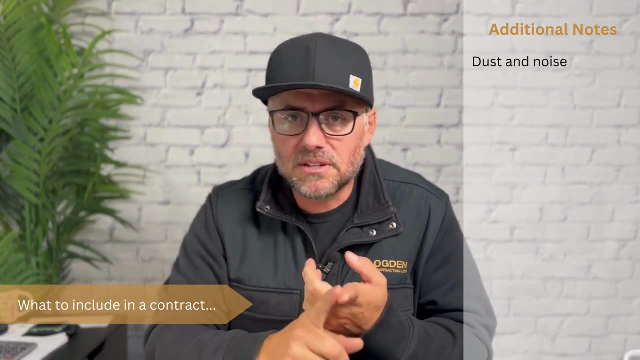 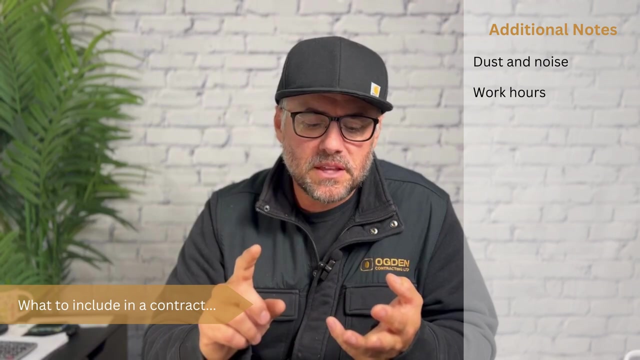 So additional notes could be anything that you want to include in there that aren't the owner's responsibilities or contractors' responsibilities, such as: there's going to be dust, there's going to be noise, holidays- you're not working holidays- the heating and ventilation like there might be, you know, when you do drywall. 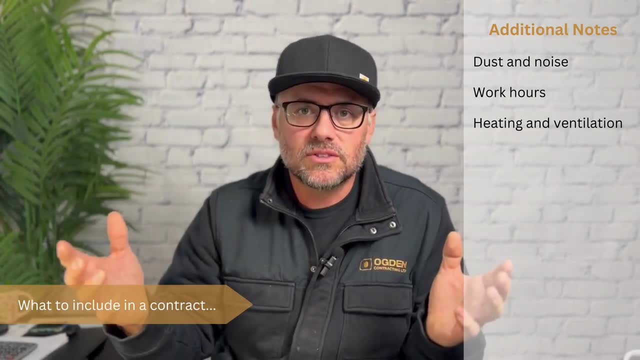 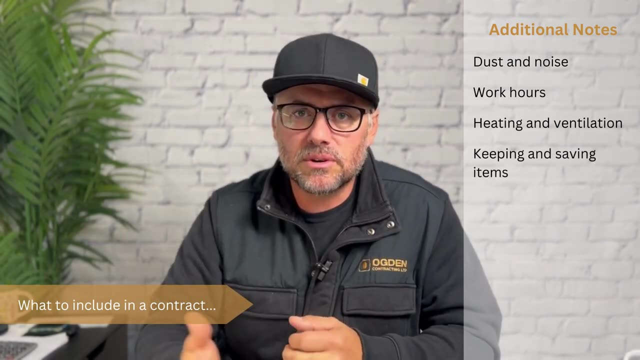 we're going to make sure that the house is heated well. So you know we need to voice these kind of things. And keeping the saved items. like I said before, it's really important to express that we're saving these items for the owner. So, and lastly, are the specific terms and conditions? 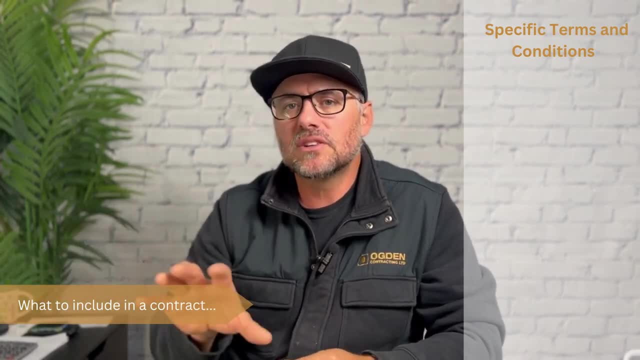 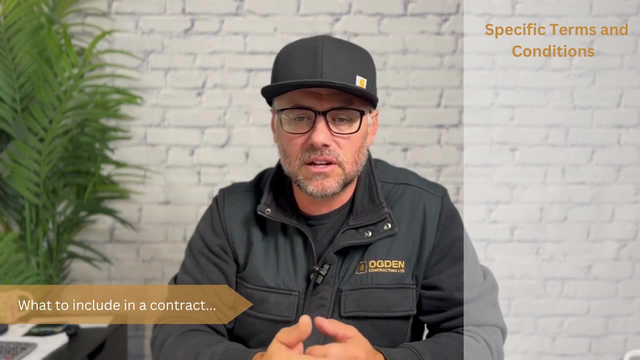 I always include this on my contract, but you should have a separate terms and conditions that you've worked through with your lawyer. But I'm going to list off just some real quick things that I include on my contract, So like the date that you're commencing work. 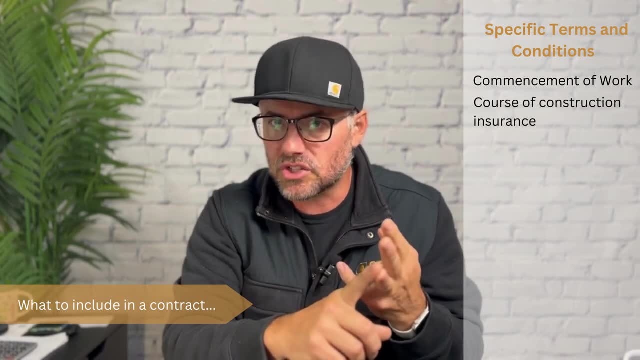 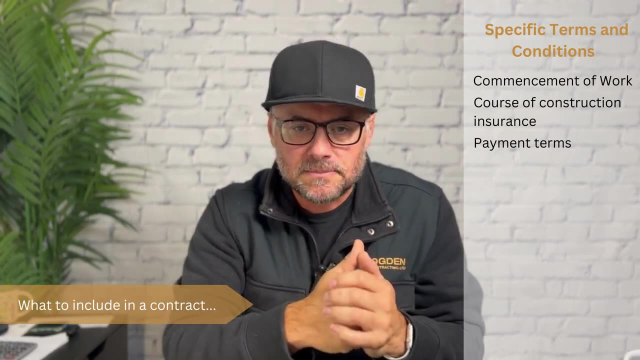 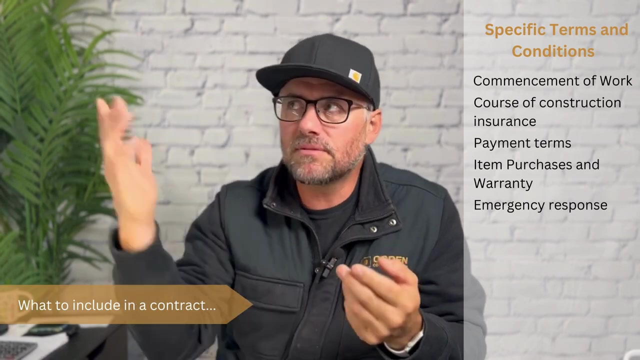 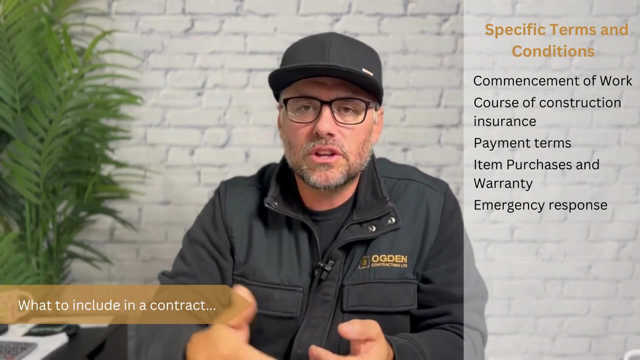 the date that you're going to be working, the course of construction insurance, your payment terms- it's always important to include those payment terms- Your items purchased and warranty items. emergency response, like what happens if the tree falls on the house or a tarp blows off or a water main breaks. What are you going to do? 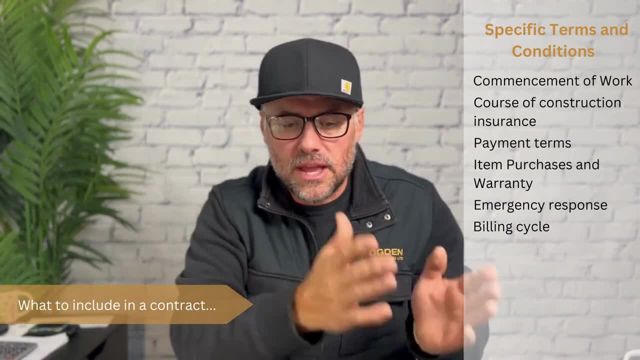 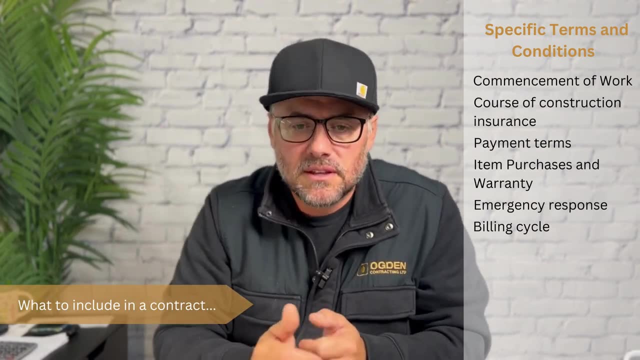 The billing cycle. you always want to include, like when you're going to be billing them so they can expect- you know they might expect- to bill once a week, once a month, bi-weekly- Your hourly rates. you always want to include your hourly rates If all of a sudden there's an extra. 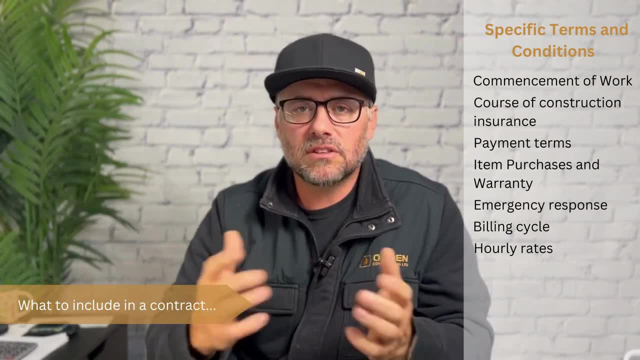 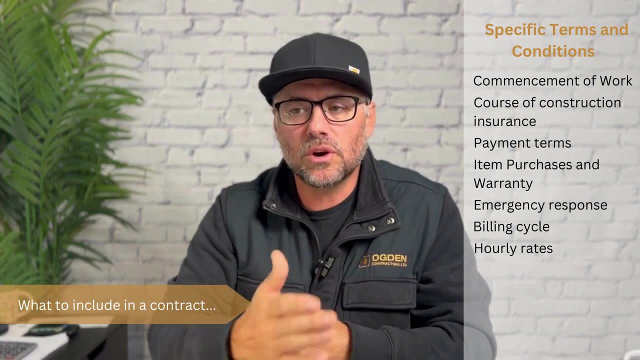 then they want to know how much they're paying by the hour. That's the other thing is extras. So what is your extras? What is your additional charges? If all of a sudden there's a change or a change work order, what is the procedure? So you want to write that in there. 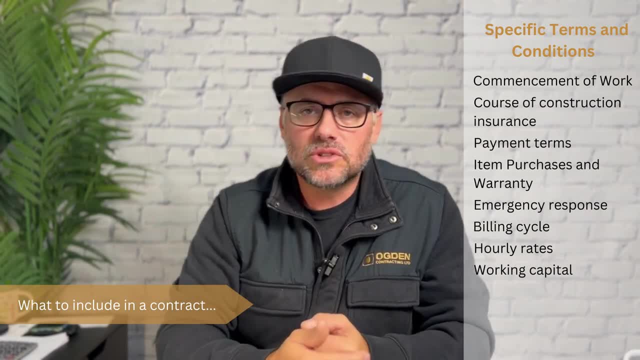 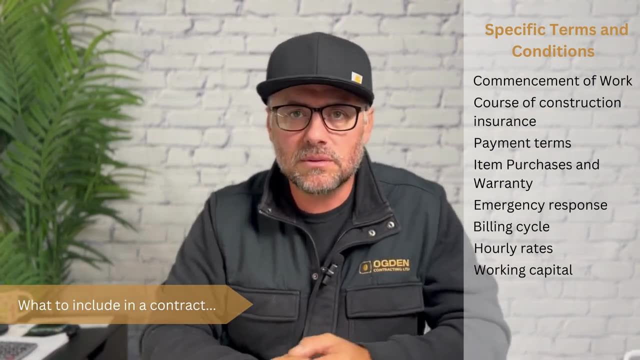 Working capital. I always talk about working capital. I don't do a job without a deposit because I like to use the owner's money for the owner's job, not my money for the owner's job. That kind of covers my butt and it increases cash flow in your company.